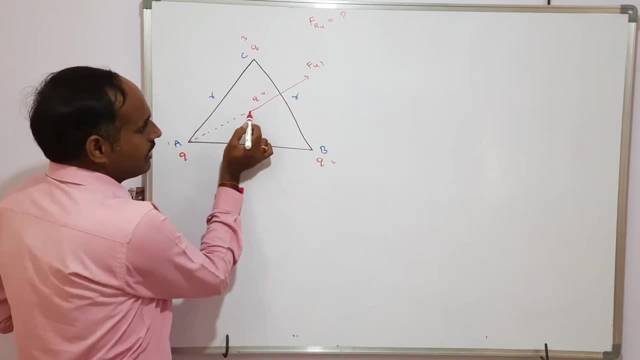 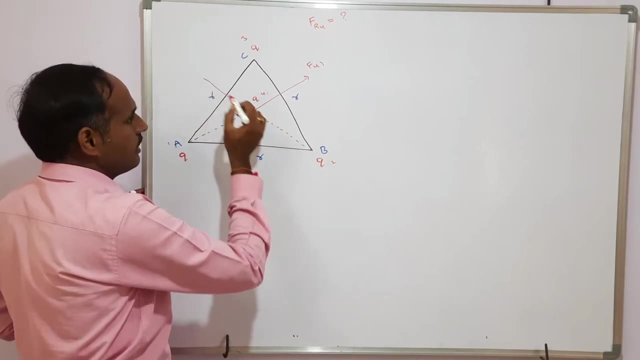 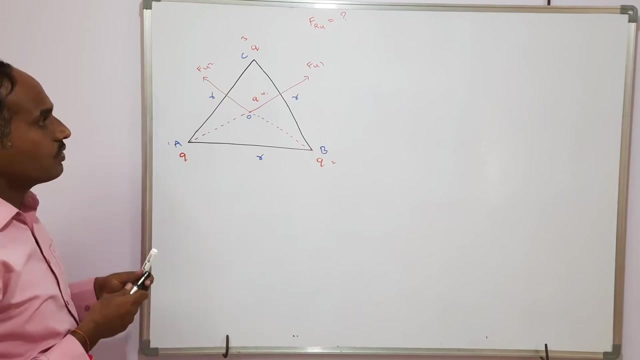 due to first And similarly coming to the force on fourth due to second. this is the line joining the fourth and second. So this is what the direction of force on fourth due to second And similarly coming to the force on fourth due to third, is the repulsive force. 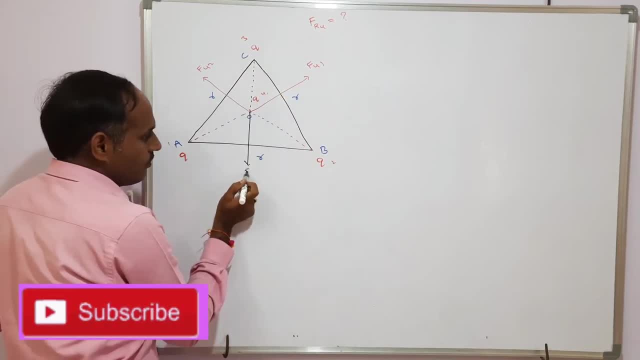 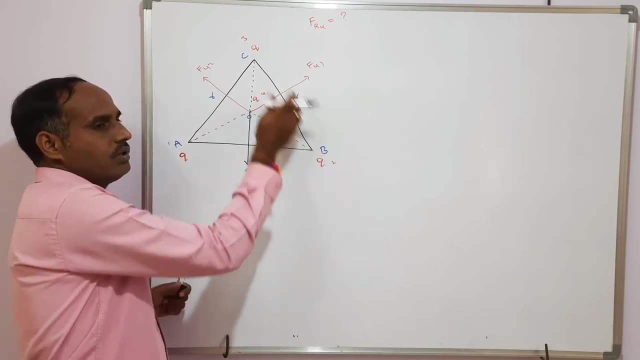 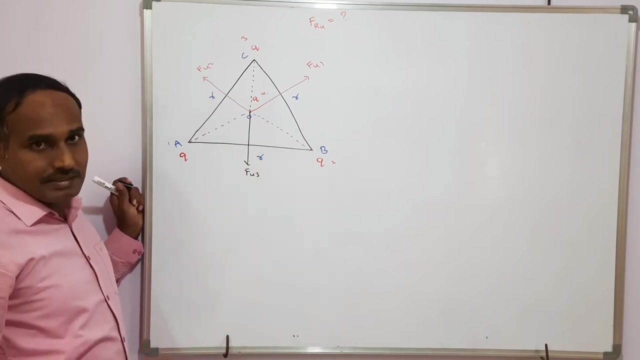 on fourth. Third is this, and the direction of force on fourth due to third is this one. So at first I am taking the direction of force on fourth due to first, second and third, And now the next thing is to write the magnitudes of all these. So if you are observing here, 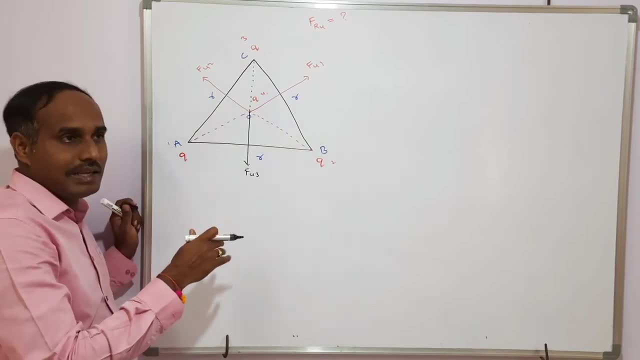 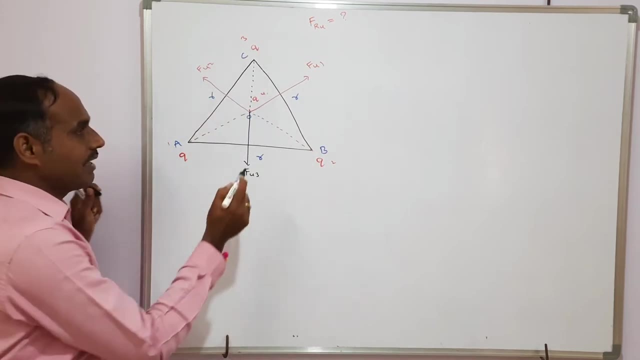 the magnitudes of one, two, three, four are same. and in the triplateral triangle the distance from centroid to the each corner is same. Each corner is same. So the distance from centroid to the each corner is same. In the Euclid triangle we can write up: AO is equals. 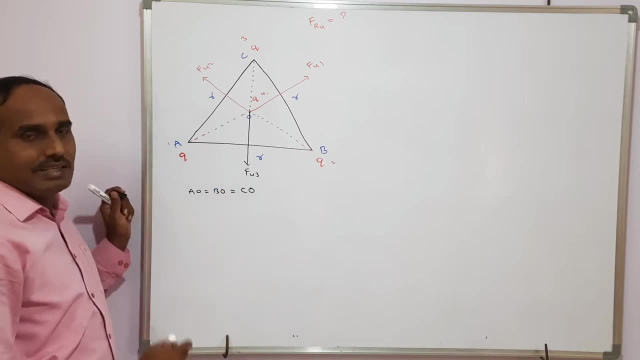 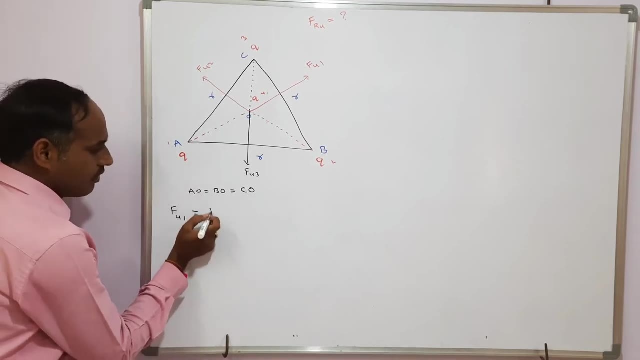 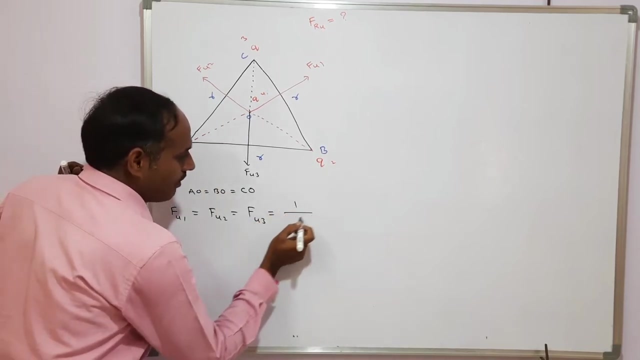 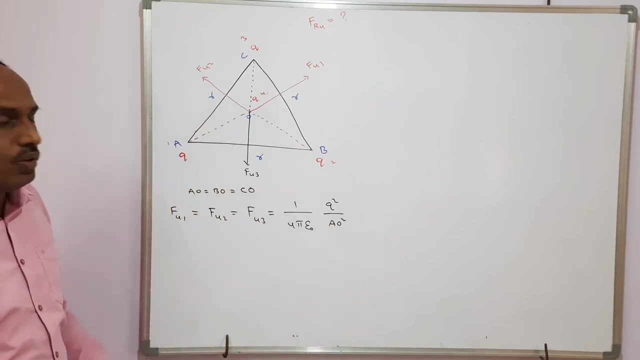 to BO, that is equals to CO and the charges are same. So that can I write here. the force on fourth due to first is equals to: on fourth due to second is equals to force due to third. This is equals to 1 by 4 pi epsilon Q square by AO square, But the AO value is unknown. 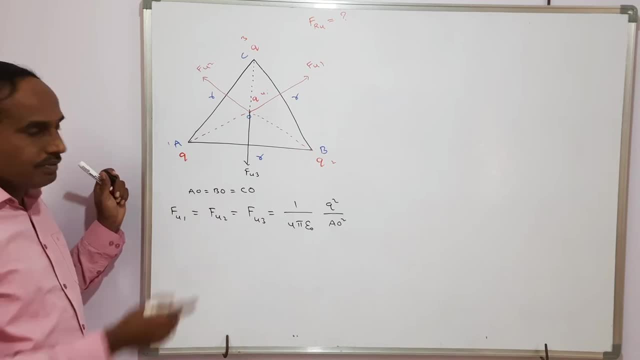 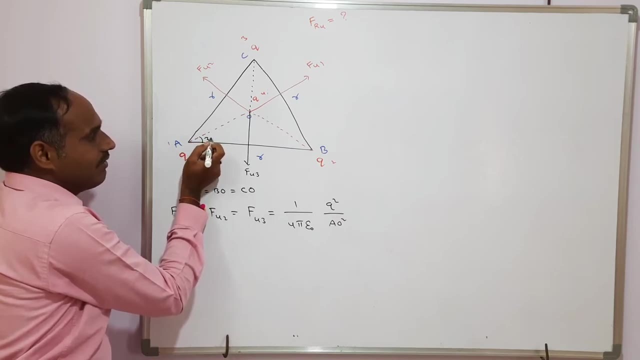 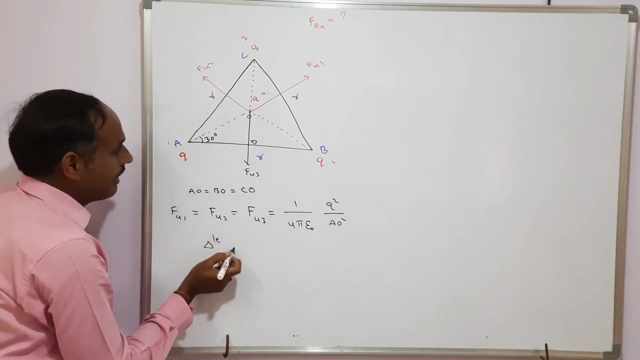 for us And to find this AO. to find this AO, what I am doing here is, as it is an angle bisector, the total angle is 60. then definitely it should be of 30 degrees, And I am coming to the point. this is supposed to be D. So consider the triangle AOD As a perpendicular bisector. 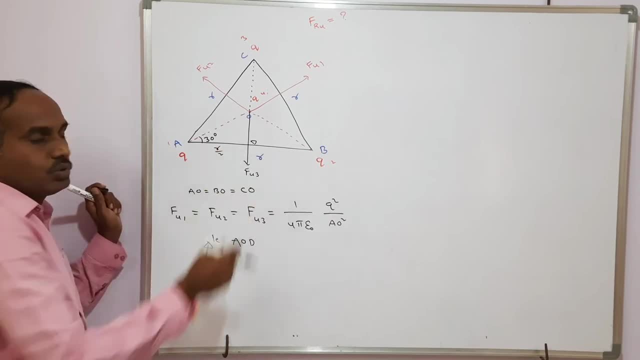 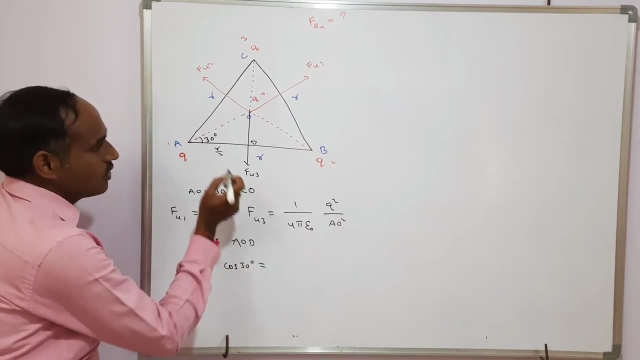 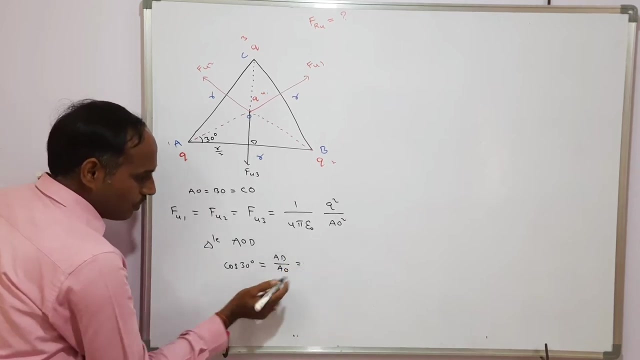 AD value definitely half the separation between the two charges, So it is R by 2.. So here can I write up cos 30 degrees. Cos 30 degrees is equals to adjacent by hypotenuse is nothing but AD, by AO And then AD value. 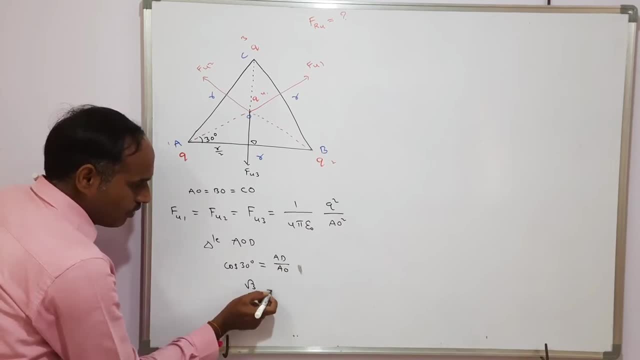 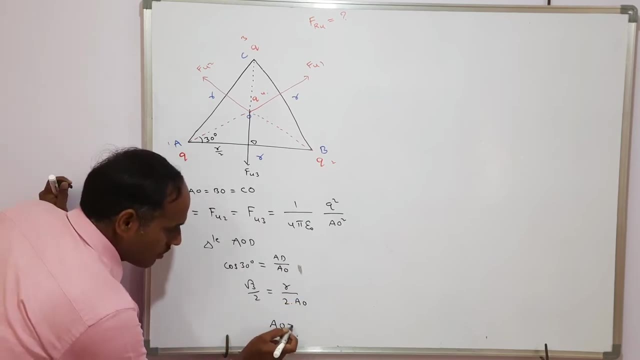 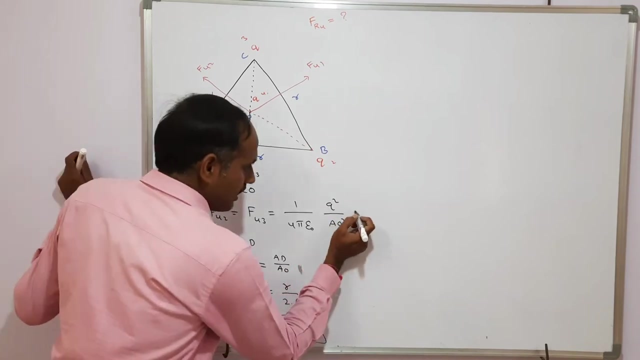 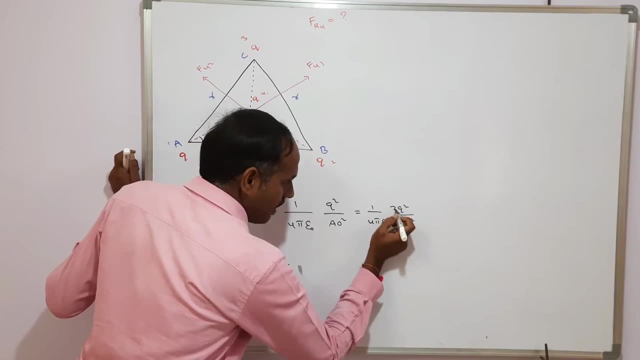 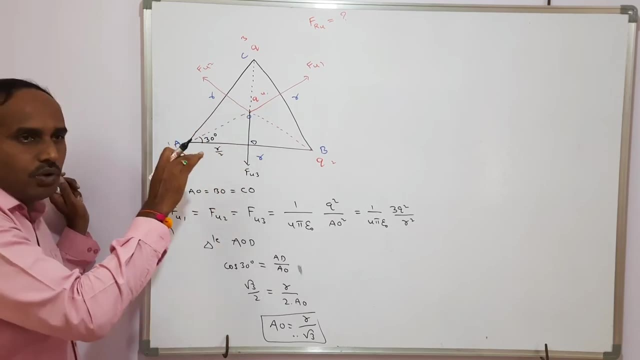 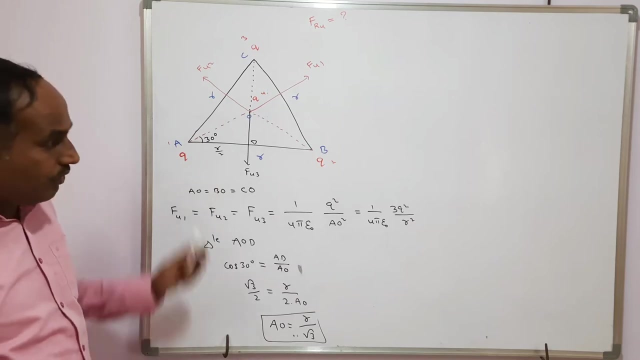 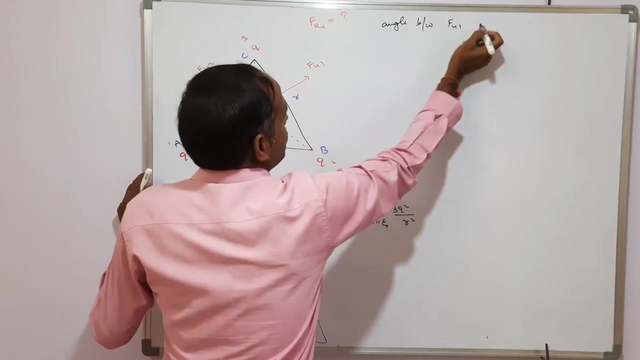 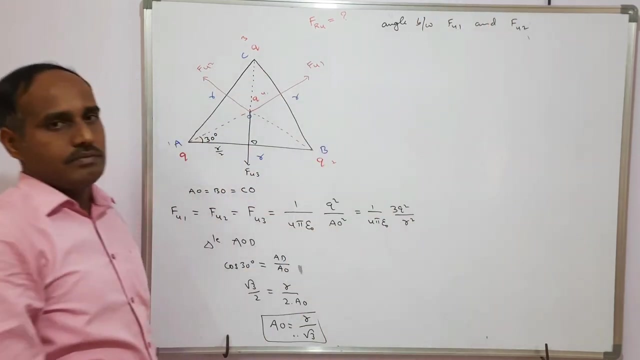 vector sum of the 3.. At first I am taking the resultant force on 4 due to first and second. After that I am coming to take a angle between force on 4 due to first and force on 4 due to second. So to get this, as it is the angle bisector, definitely it should be of 90 degrees. 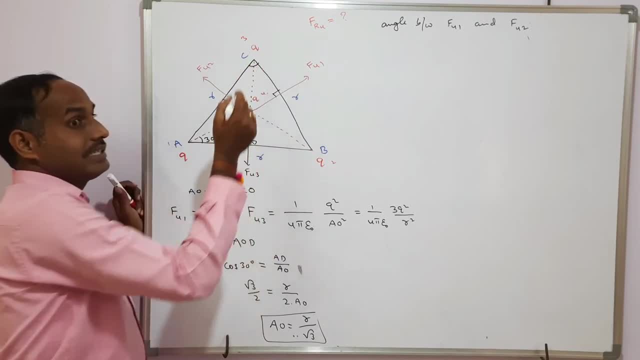 and here it is also be 90 degrees, and we know this is a 60 degrees. So in any quadrilateral the sum of the angle should be 360 degrees. So 90 plus 91 is equal to 60 degrees. So this is equal to 60 degrees. So in any quadrilateral the sum of the angle should be 360 degrees. 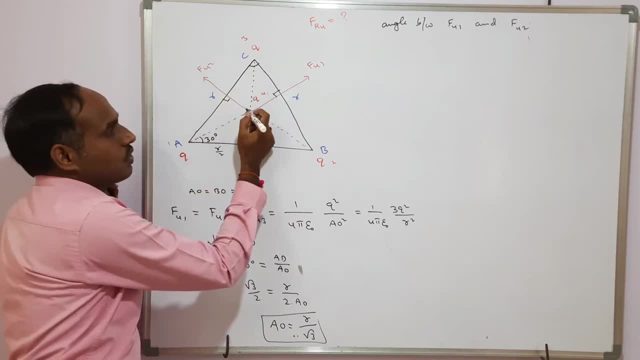 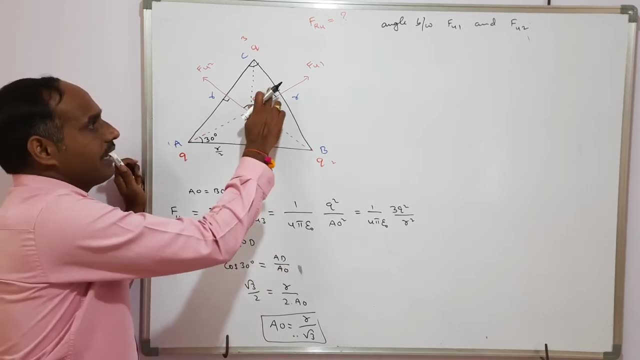 So this is equal to 90 degrees, at which I have taken the value 90 plus 90, 180 plus 60, 240.. So this angle should be of 120 degrees. Denis Quart students. So here this is 90 and is the 90, 180 plus 60, 240, and in any quadrilateral that sum of the angle should be 360.. So based 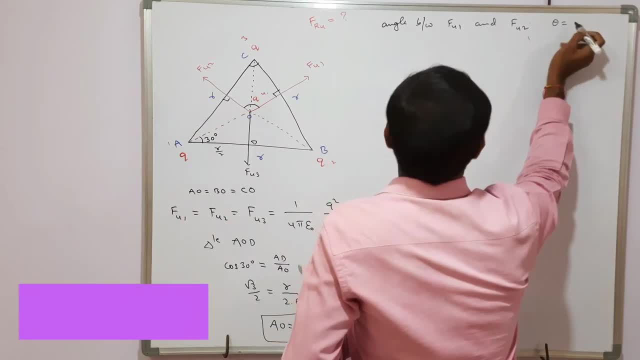 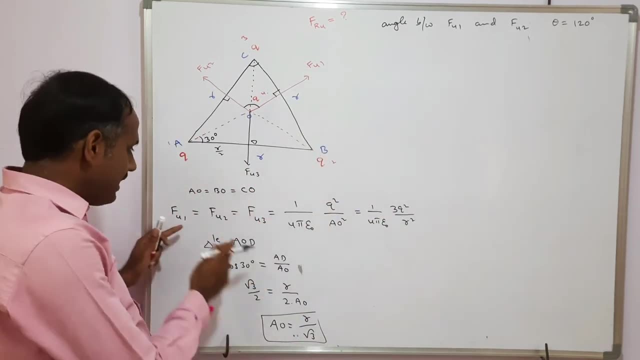 up here. I can write theta as this, theta as 120 degrees here, So whether the angle is 120 degrees and the 2 magnitudes are equal, So that the net force is equal to 0 today. I already explained this point like that. 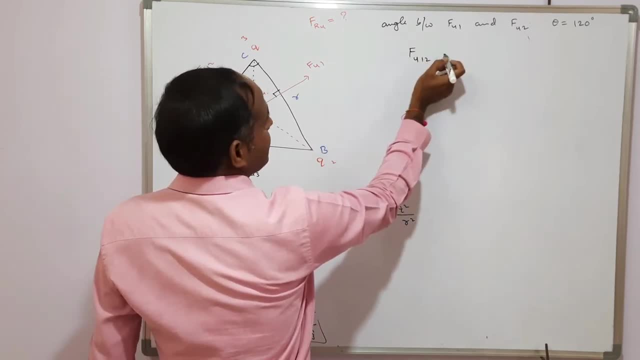 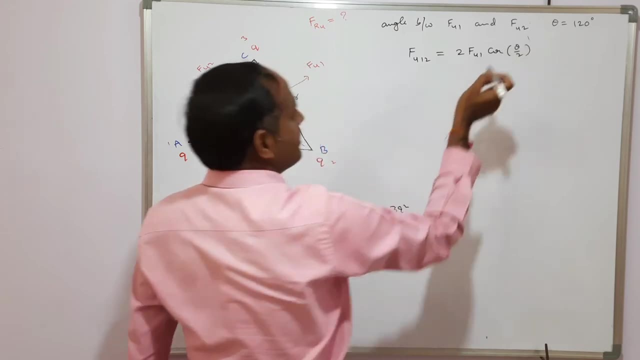 So when you call into population H with a function it is same thing. So that in arrow to force on fourth due to first and second can be written as: 2F41 cos theta by 2 is the generalized formula from again, special case of parallel ground of vector, So that here: 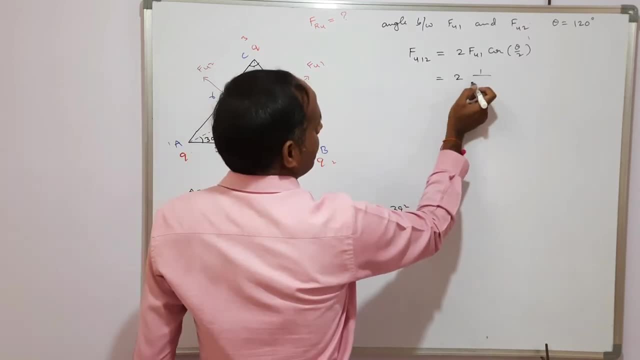 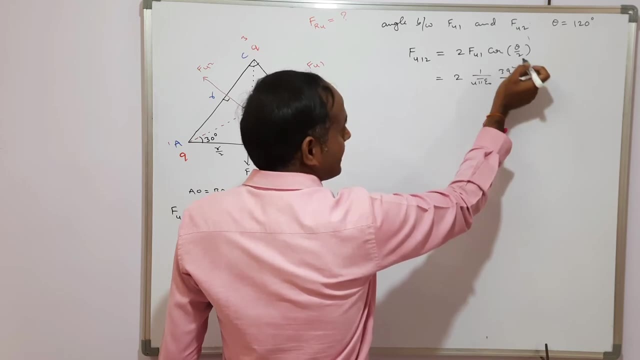 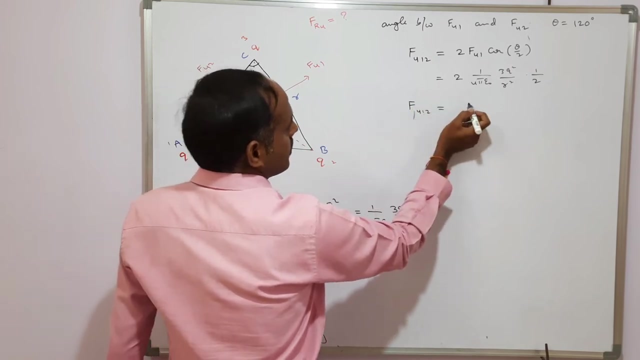 you can write 2 into F41 is 1 by 4 pi epsilon. 3Q square by R. square into cos theta by 2 is a cos 60, cos 60 is a 1 by 2.. So that you will get: F412 is equals to 1 by 4 pi epsilon.